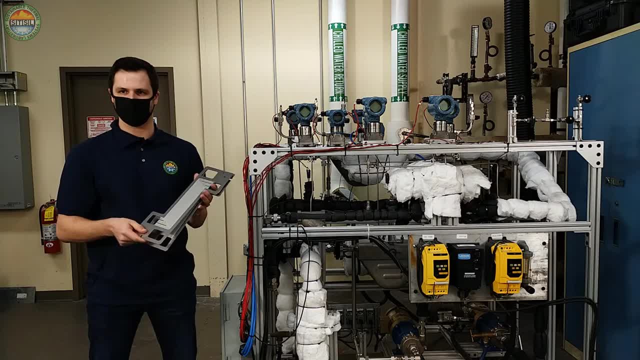 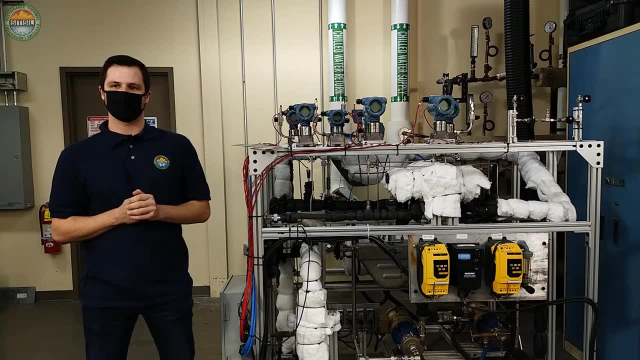 Then the sheets can be stacked on top of each other to provide the amount of heat duty required. This is the test facility that we developed to validate the microchannel heat exchanger design. The test facility has multiple loops. They carry the hot, boiling and cold fluids that simulate the primary and secondary coolants in the actual reactor. 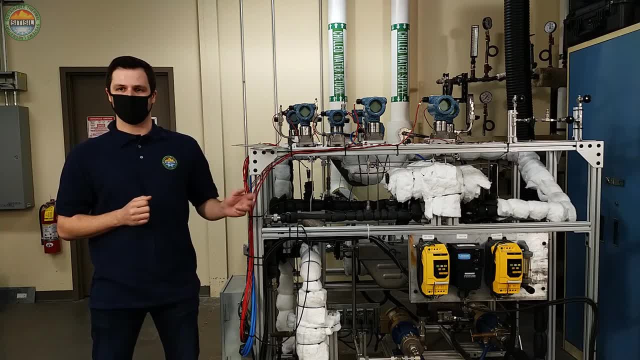 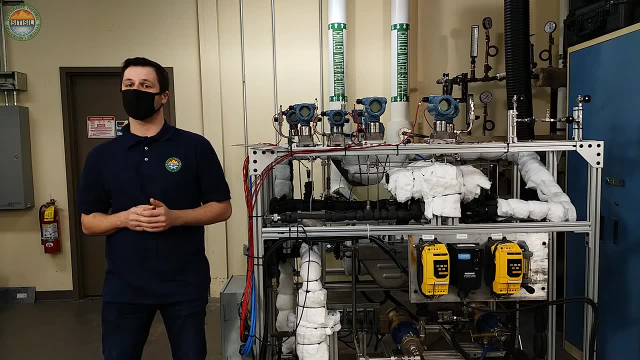 This test facility has temperature, pressure and flow rate instrumentation to quantify the heat duty and pressure drop for a representative microchannel heat exchanger test section. We have performed a wide range of tests with both single-phase and two-phase flow of the secondary fluid. 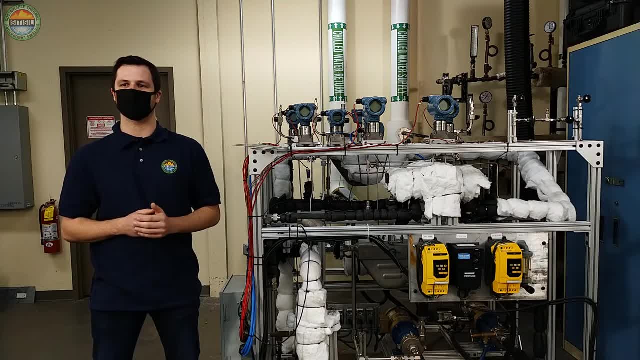 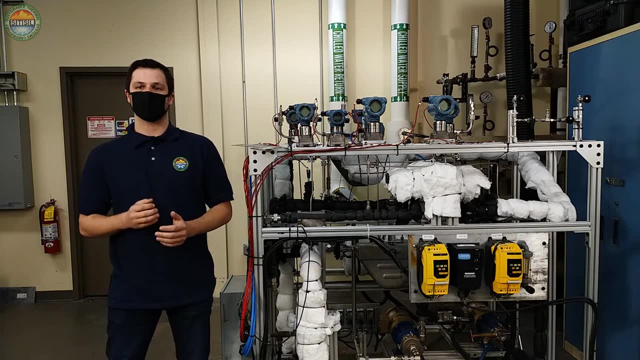 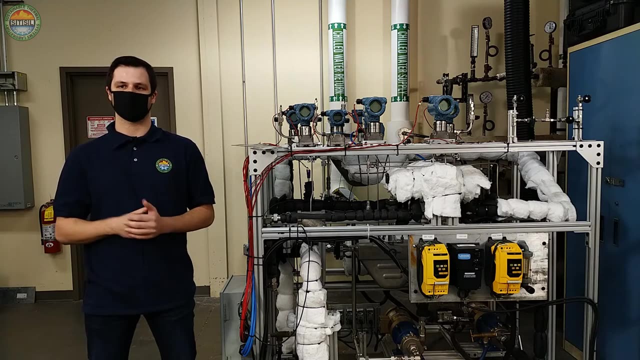 The results from our experiments show that the microchannel heat exchangers can achieve the power densities required for the reactors with integral primary coolants. Another area of focus is on advanced high-temperature reactors. These reactors use molten salt as the coolant at roughly atmospheric pressure instead of high-pressured water. 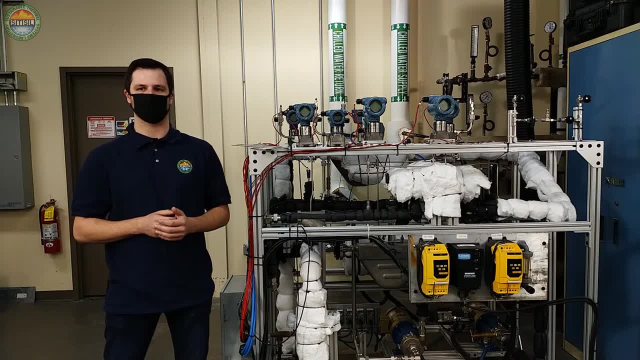 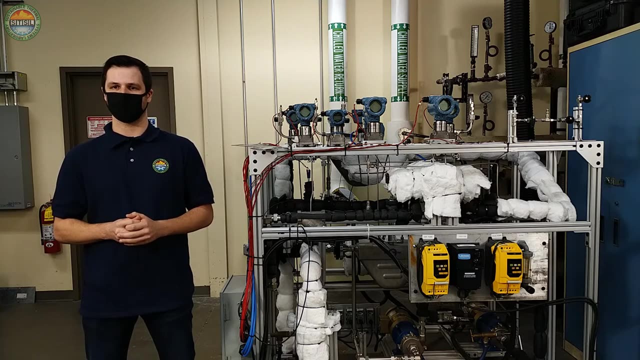 This makes them inherently safer and more efficient than light water reactors. The hydrodynamics and heat transfer for the geometry are not well understood for the plate-type molten salt reactors. This study will help in understanding the effect of different coolant channel design features on the thermohydraulic performance of the reactor core. 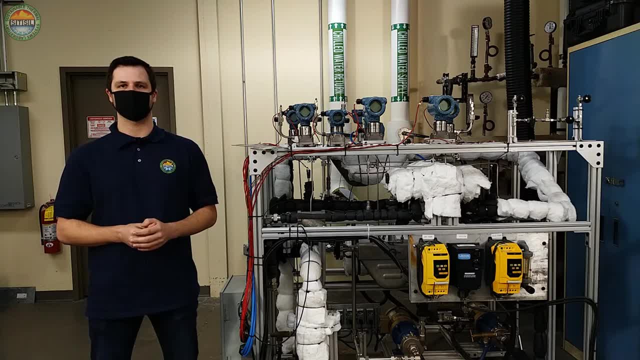 both during normal operation as well as postulated accident scenarios. In addition, the correlations developed from this work will assist benchmarking efforts of safety evaluation codes being developed by the NRC for licensing advanced nuclear reactors. In these experiments, local heat transfer coefficient and friction factor are investigated for flow through plate-type geometry. 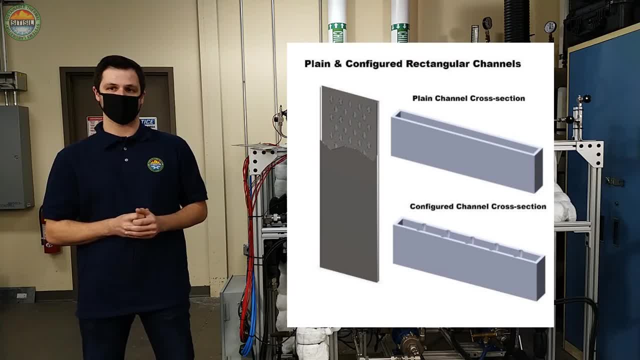 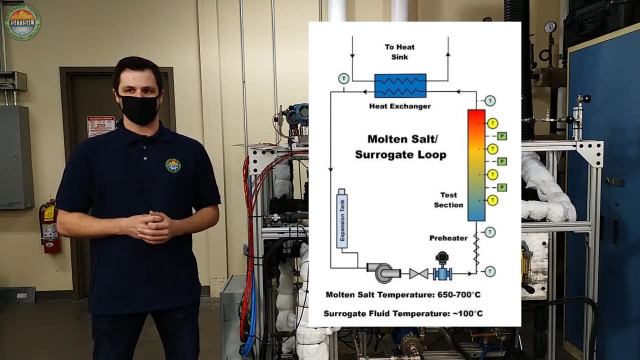 In addition, a channel with dimple features is investigated to characterize and quantify the heat transfer enhancement for heat transfer. This is done in both normal operation as well as accident scenarios. For the experiments, a commercially available surrogate fluid that simulates the molten salt properties is used. 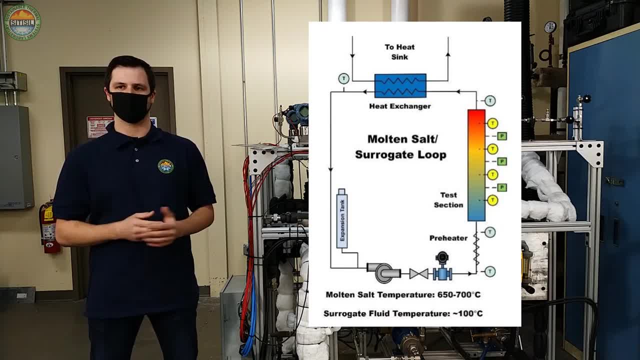 This fluid flows through a test section that consists of a rectangular channel to simulate the plate-type geometry, and the channel is heated electrically to simulate the fuel strength in the reactor. Instrumentation that measures temperature and pressure at axial locations along the channel are used to collect data that is applied for the calculation of the local heat transfer.